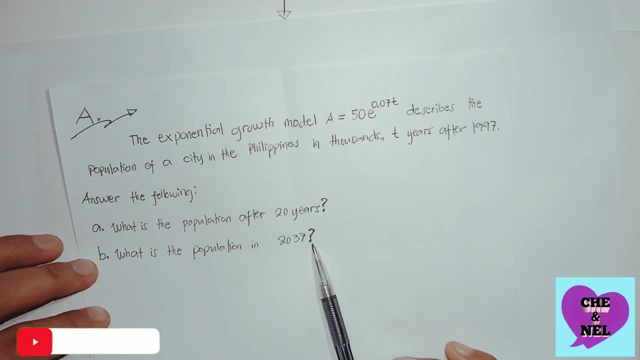 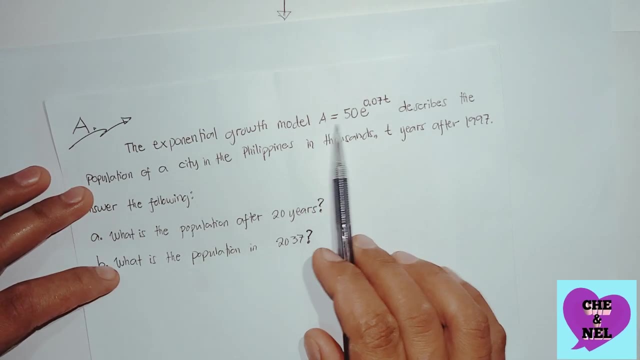 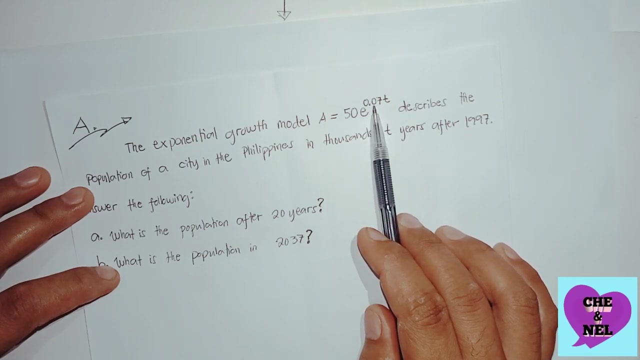 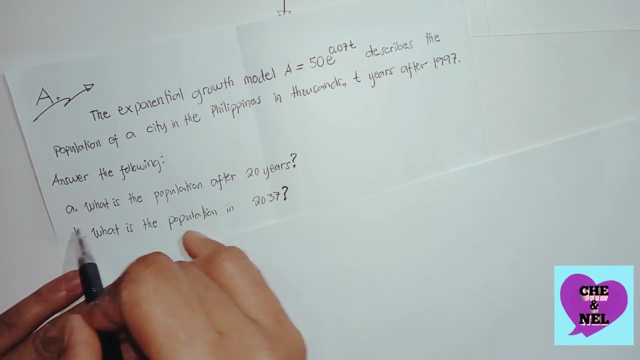 Letter B: what is the population in 2037?? Okay, so we all know that in our growth model here we already have the value of r, which is equal to 0.07.. Okay, Okay, So let's take a first problem, letter A. So what is the population after 20 years? 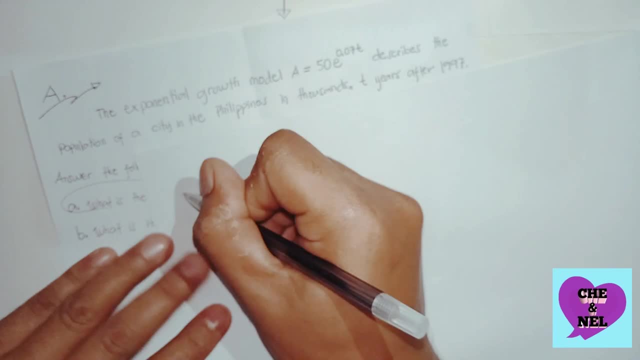 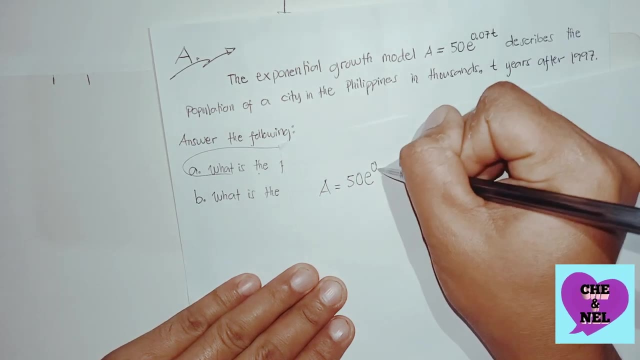 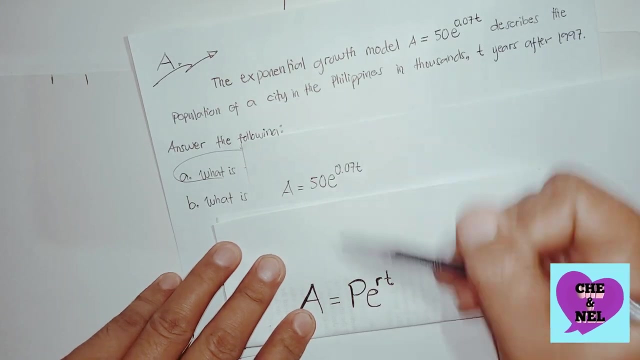 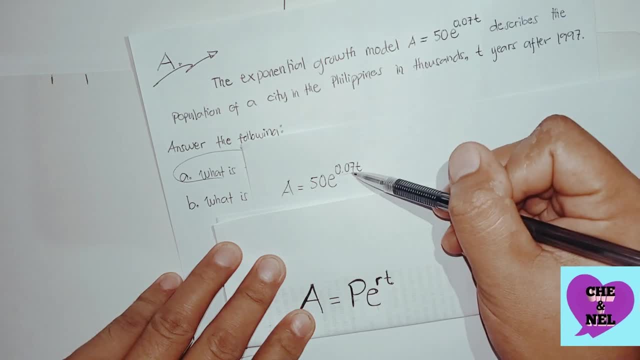 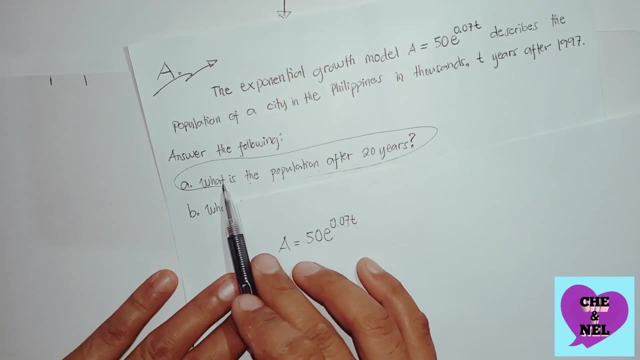 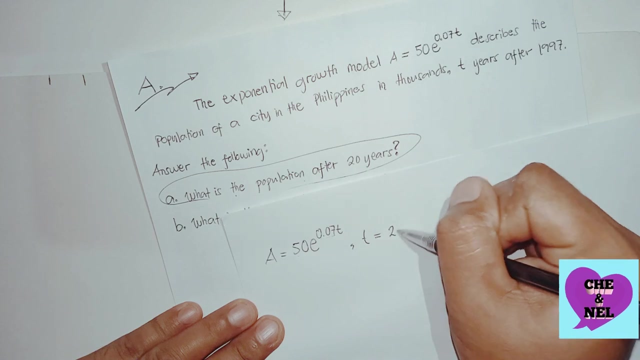 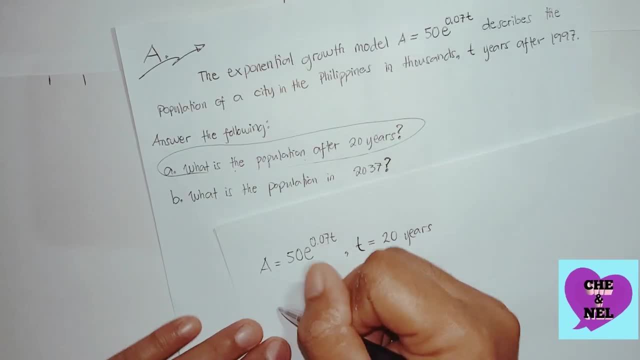 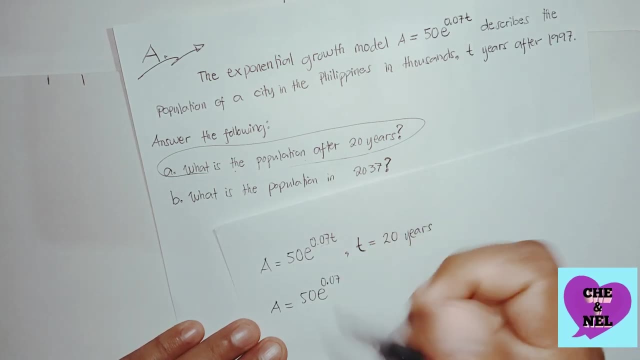 t is time, Okay, So to continue. we have here 50 a raised to the power of 0.027.. There we go. Okay, Okay, 0.07, just copy, then insert the value of d, the 20 years, which is 20, then simply continue. we have. 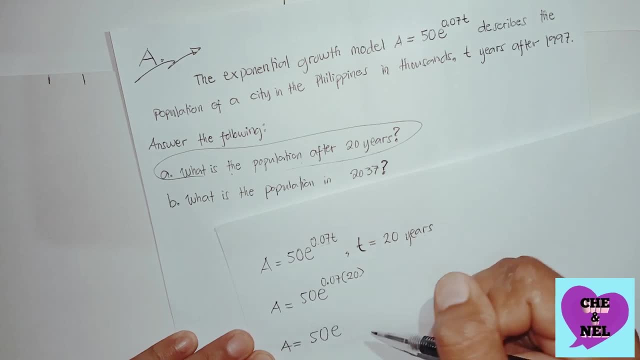 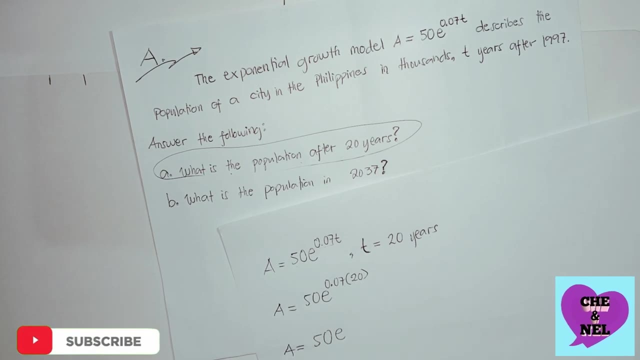 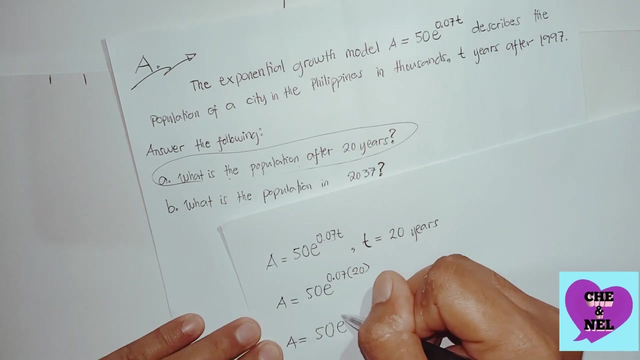 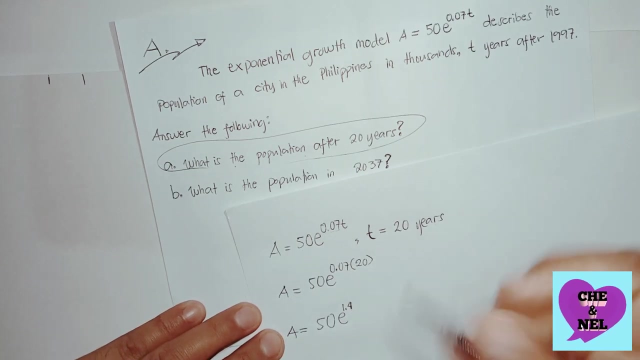 here 50 e raised to the power of 0.07 times 20. okay, so 0, 0.07 times 20 is equal to 1.4. so the exponent of our Euler's variable is equal to 1.4. okay, so now let's find first the value of. 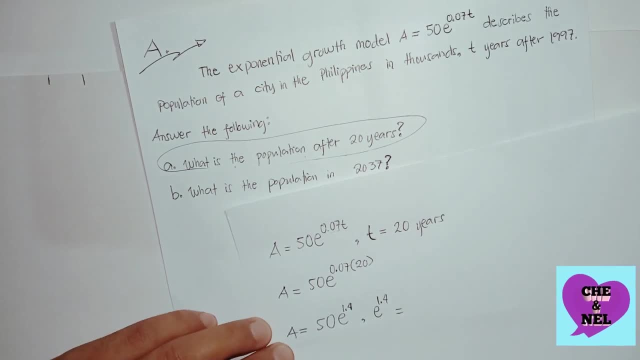 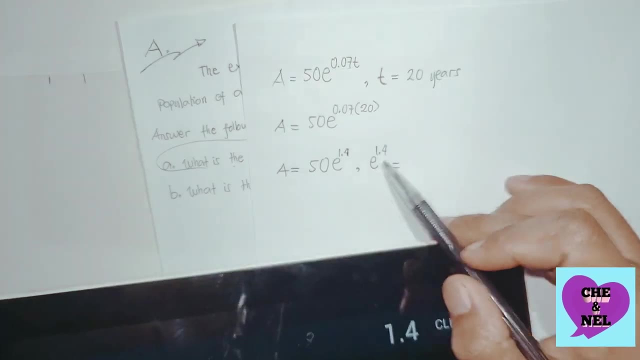 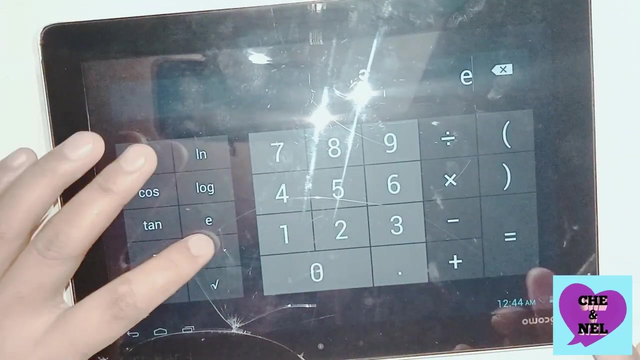 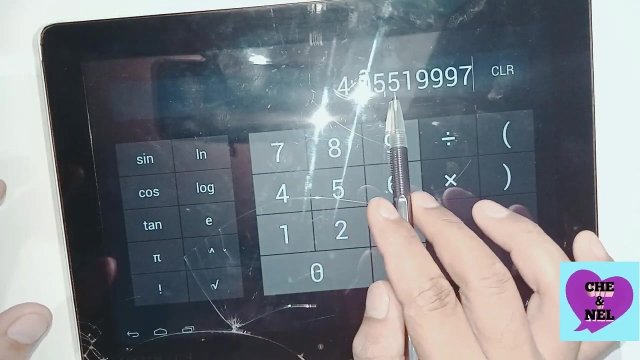 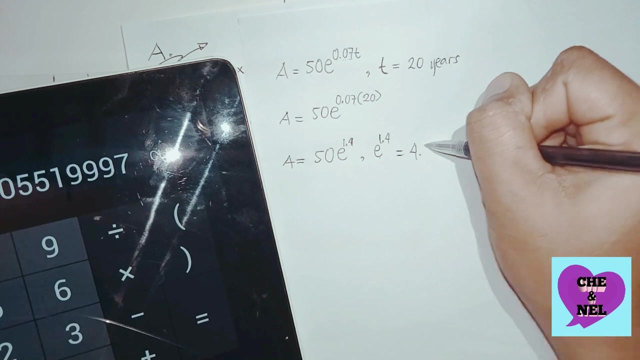 a raised to the power of 1.4. we can use here the calculator for us to have the value of a raised to the power of 1.4. so now we have here: a raised to the power of 1.4 equals 4.055. okay, so the value of a raised to the power of 1.44 is equal to 4.055. 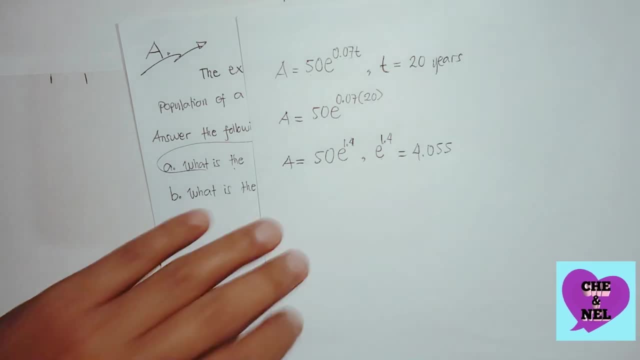 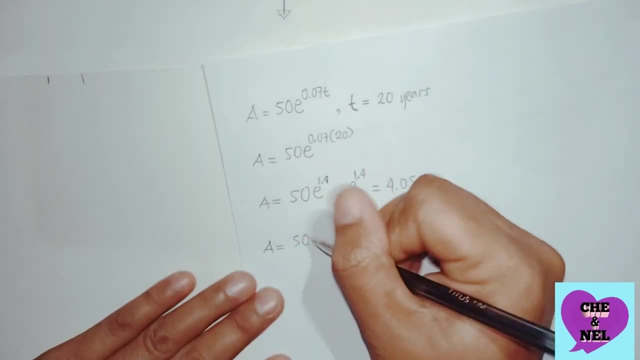 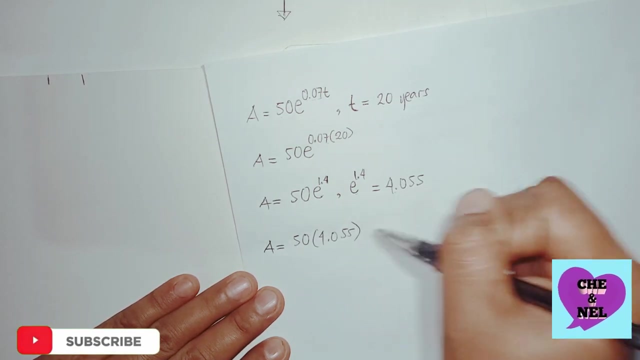 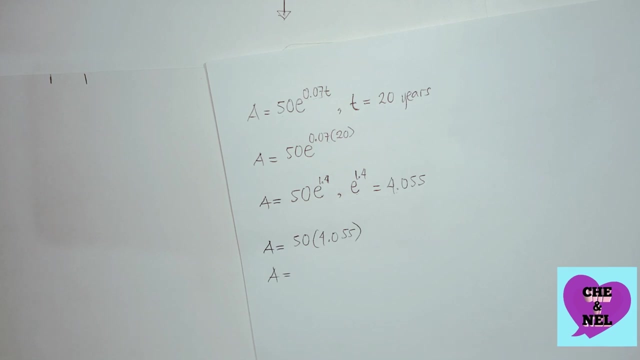 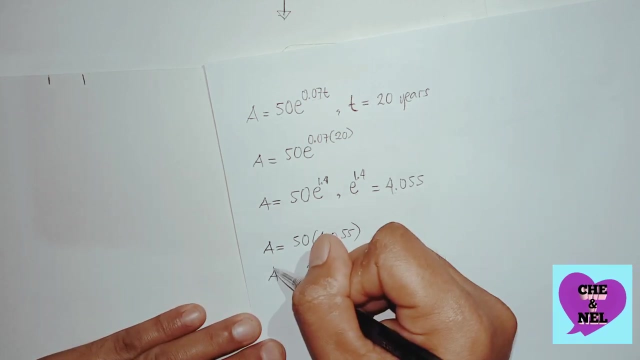 okay, so thank you, calculator. then we have here: a is equal to 50. what's the value of a to the 1.4 is 4.055, 0.055. okay, so 50 times 4.055 is equal to that is 202.75. okay, we have now the value of a. 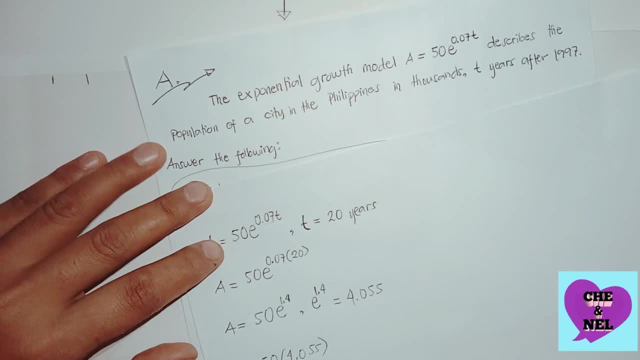 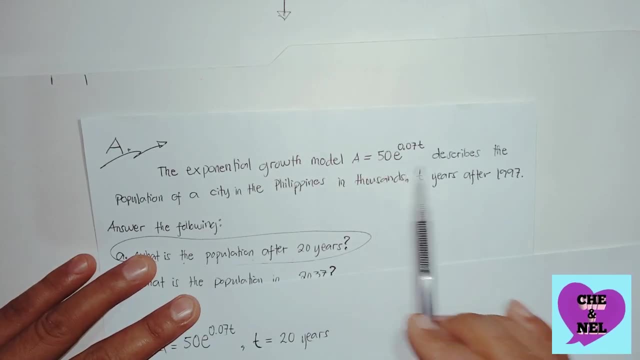 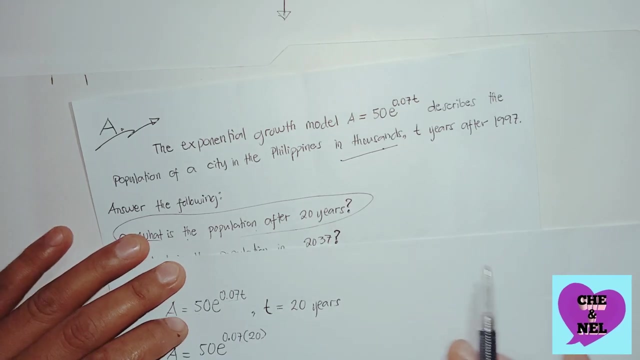 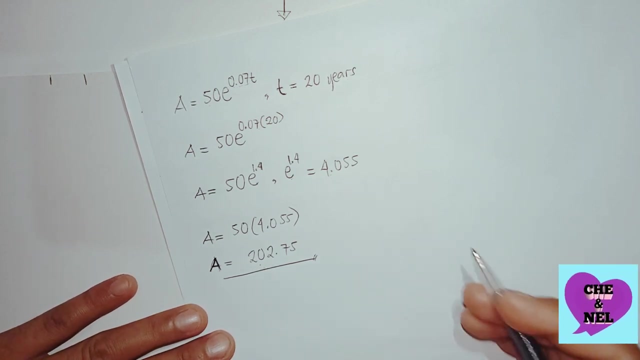 then let's go back to our main problem, i mean main statement. the exponential graph, model A is equal to this. one describes the population of a city in the philippines in thousands. okay, the population should be in thousands. that means to say: that means to say this population here should be multiplied by this number here should be multiplied. 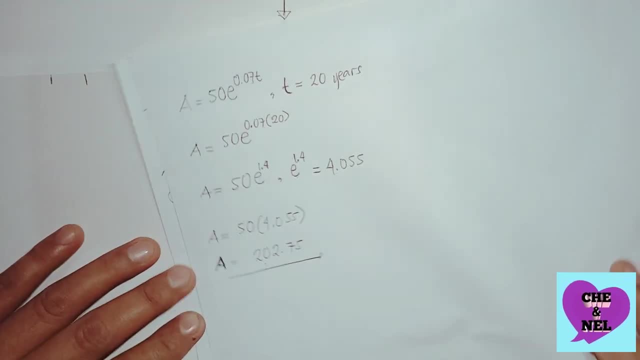 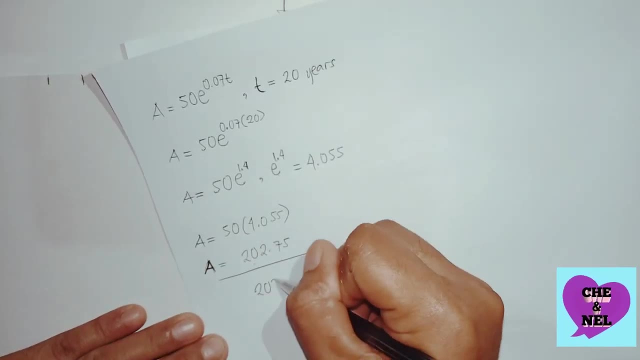 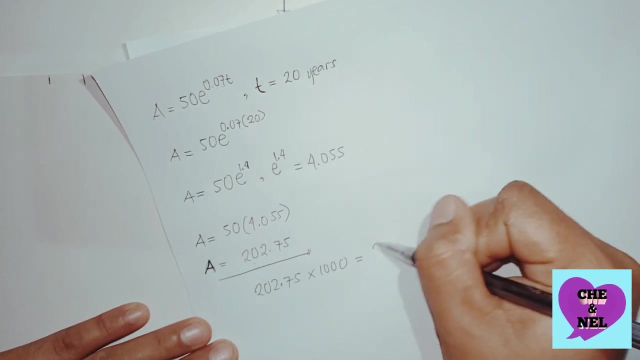 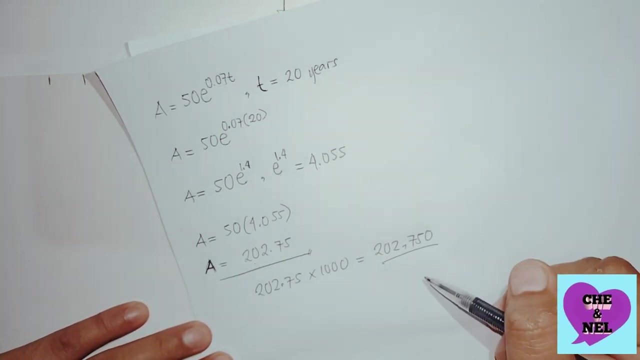 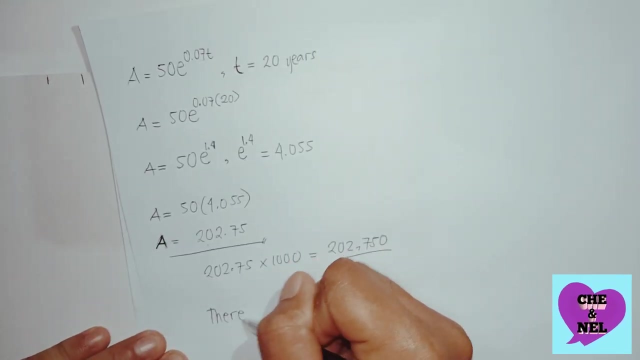 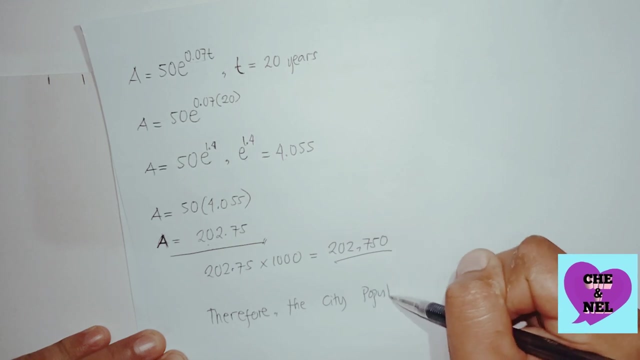 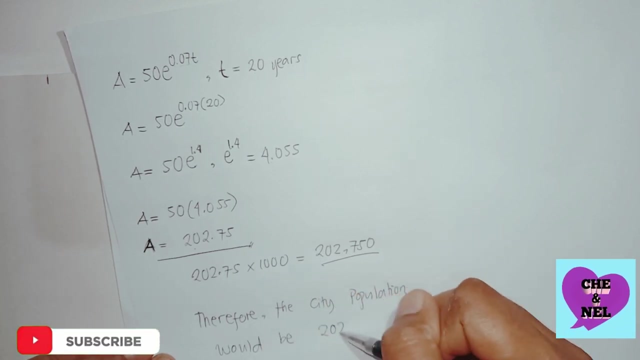 by one thousand, because, based on our original statement, we have here in thousands. so i think that's clear. so we have here five hundred two, 175 times 1000, that is to say we have 202,750 people. okay, so let's make this final answer. we have here. therefore, the city population would be: 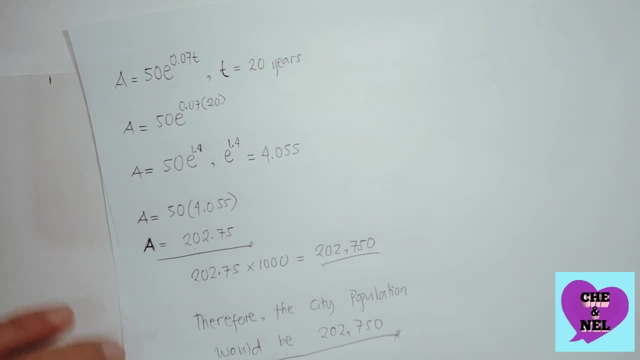 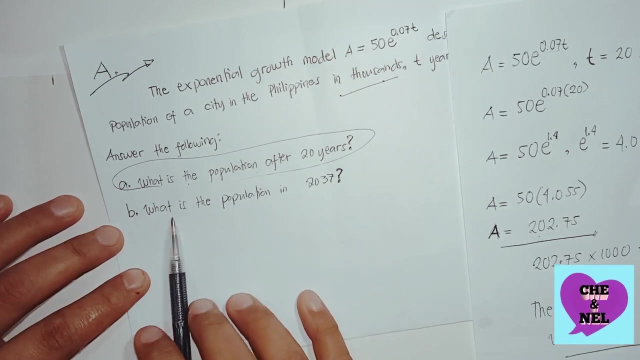 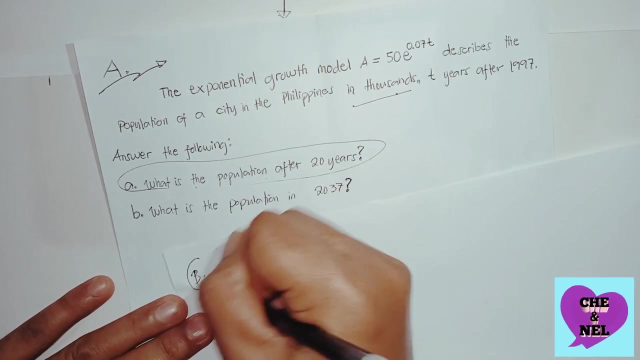 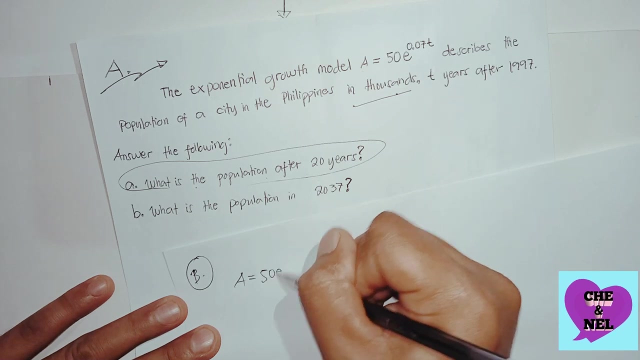 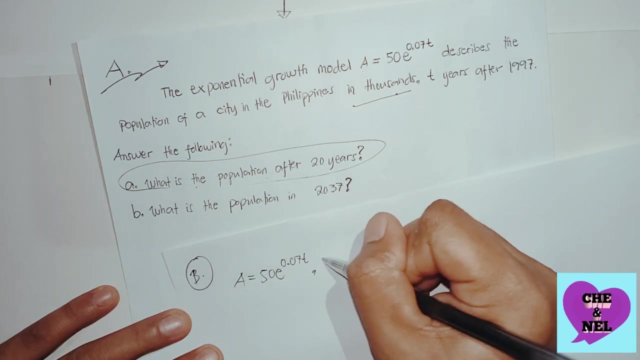 202,750. so this is now our final answer. so we are done with letter A problem. and then let's now take out the letter B problem. okay, so in our letter B we have: okay, so we still have to copy this one copy: 0.070. okay, so at this point of time we will now know the value of our time, our t. 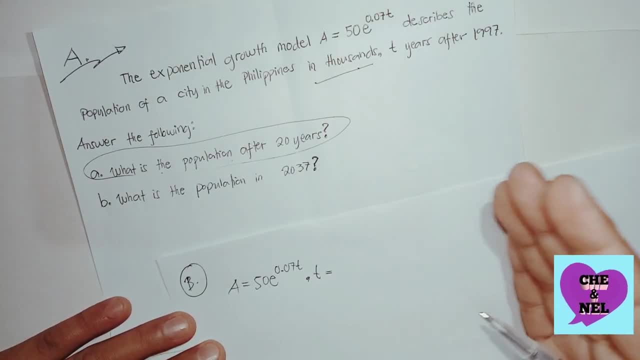 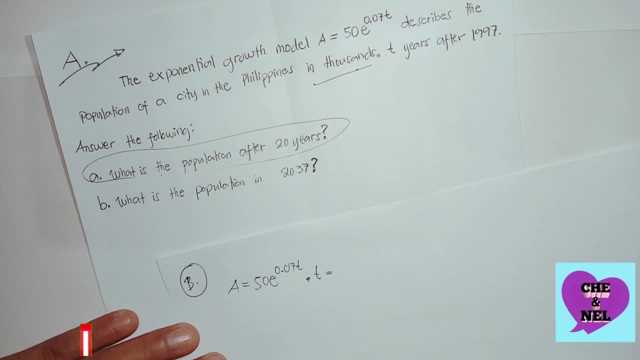 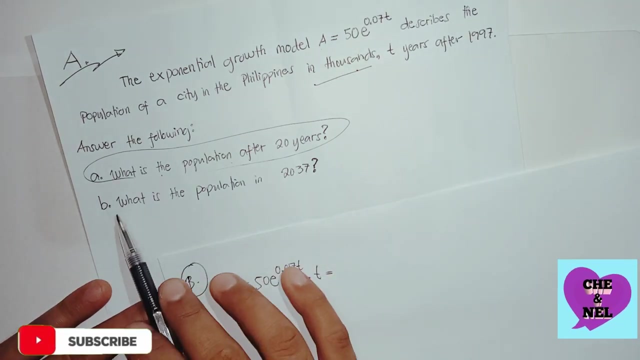 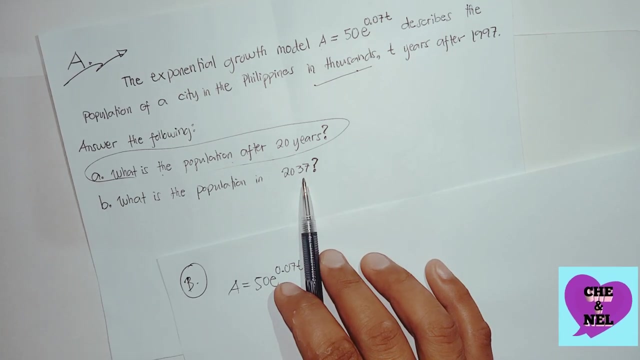 t. so how are we going to know the value of t? what particular way we're going to apply to find the value of t? it is very simple, because we have here at the years after 1997, then our problem be: what is the population in 2037? so this certain year here is more advanced. compare here. so we have 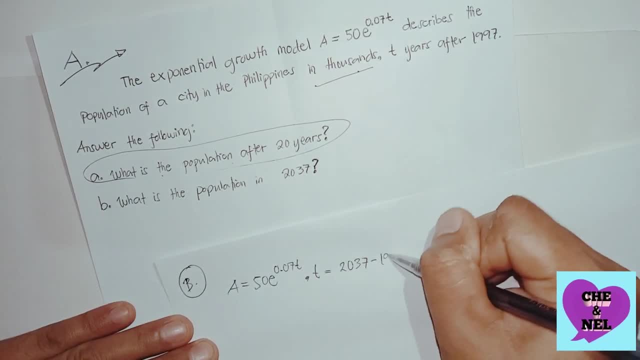 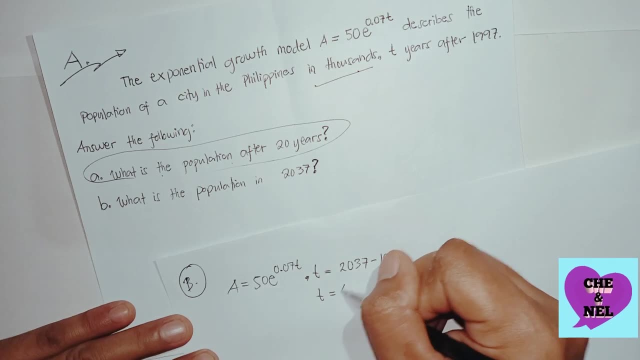 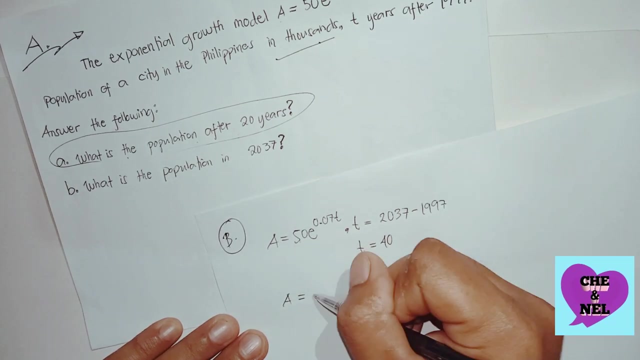 here 2037 minus 19, 1997. so the value of t simply should perform the difference. then the value of t is equal to 40. let's continue. so, to continue the solution, let's simply copy 50, a raised to the power of. 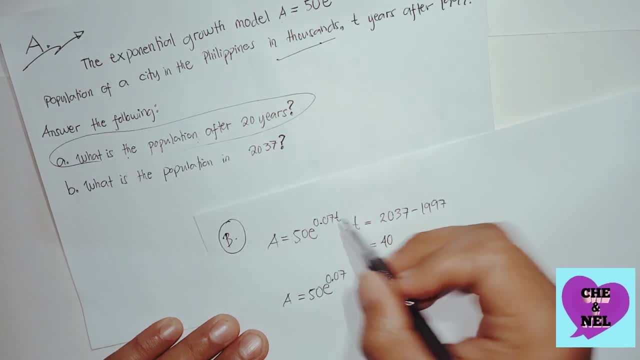 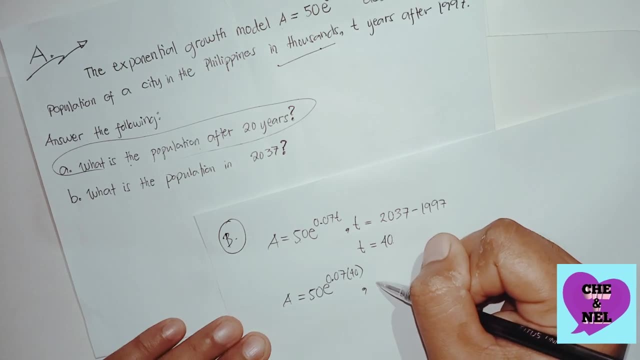 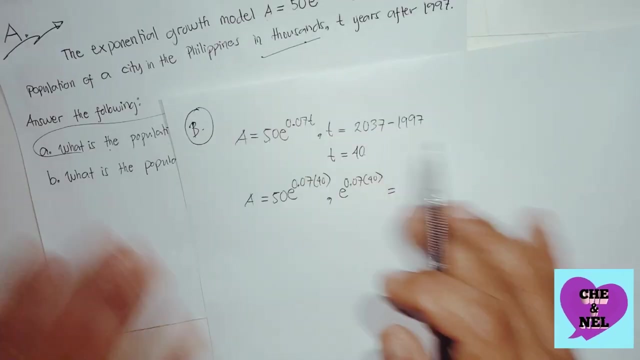 copy: 0.07 t. what's the value? of t is 40, so 40 okay. so we have here 8, the power of 0.07 times 40.. Let us first multiply: 0.07 times 40 is equal to 2.8.. 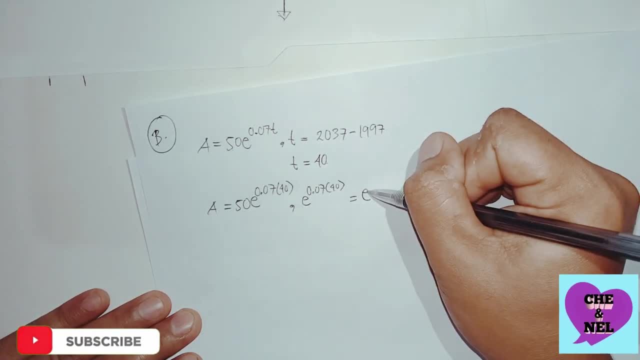 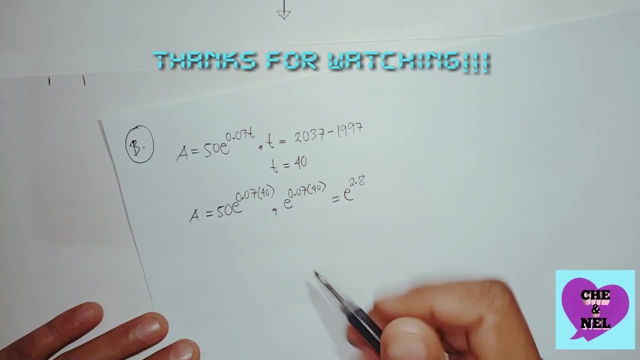 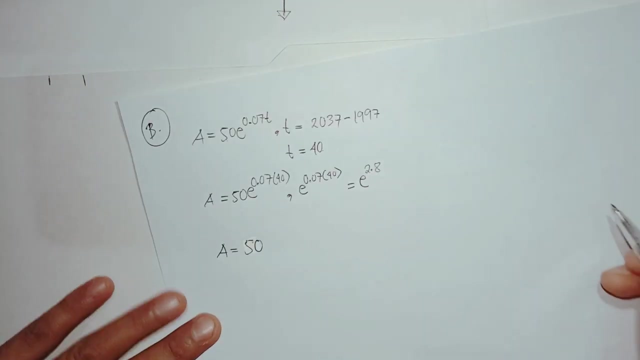 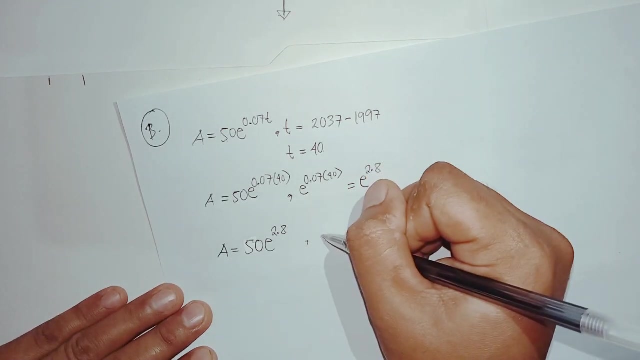 That means to say, the exponent of our Euler's variable is 2.8.. Okay, that simply means that A is equal to 50E raised to the power of 2.8.. Okay, let's know now the value of our E to the power of 2.8. 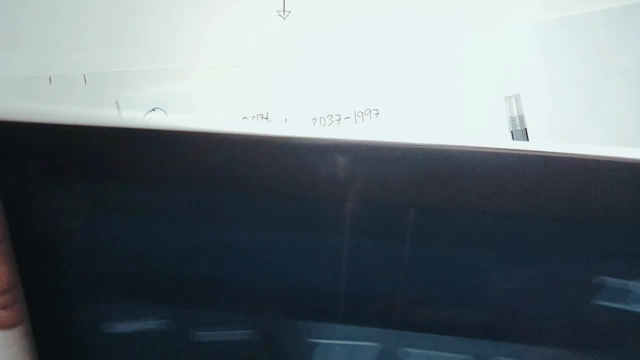 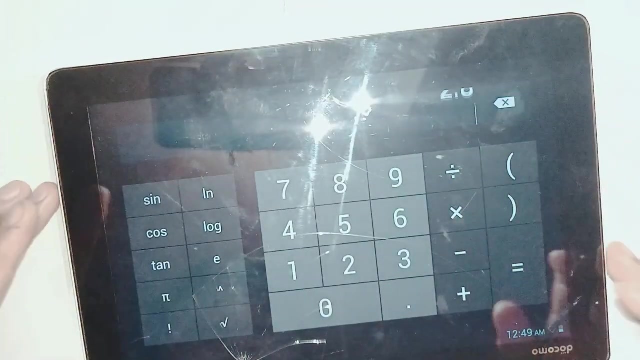 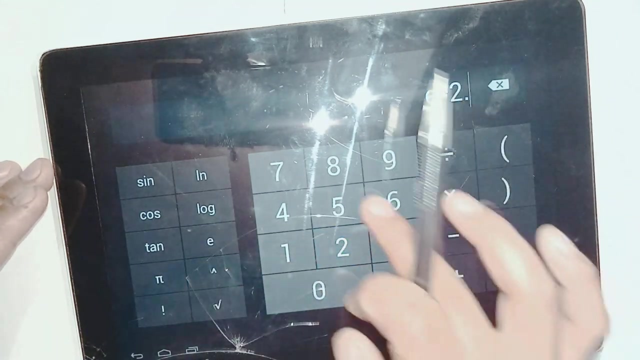 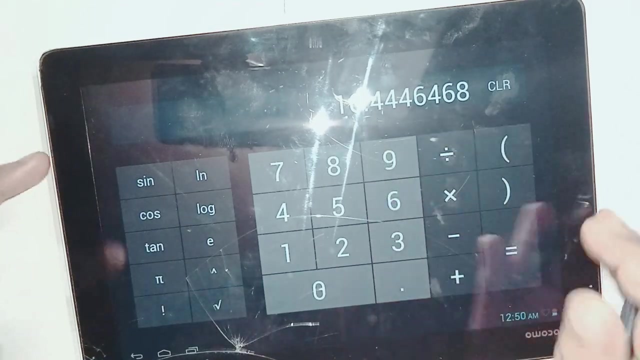 Using again the calculator, we can have the value of A to the power of 2.8, so we have here- Please excuse, before you comment- one raised to the power of, raised to the power of 2.8. so it calls 16.445, 16.445. thank you, calculator. 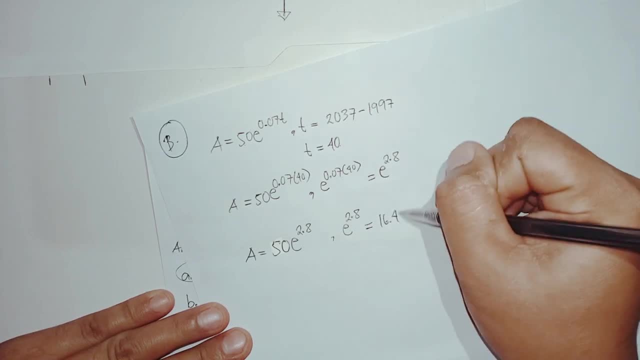 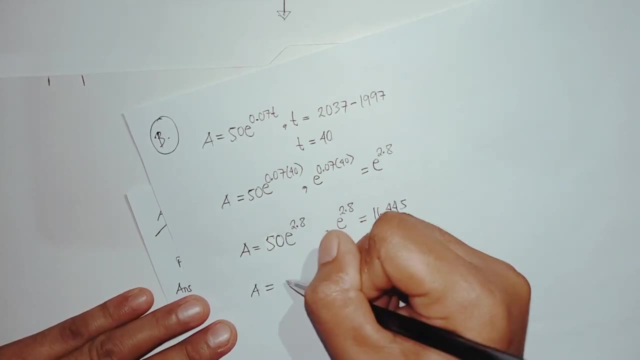 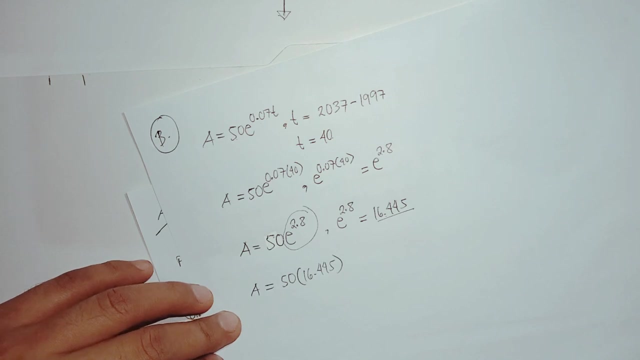 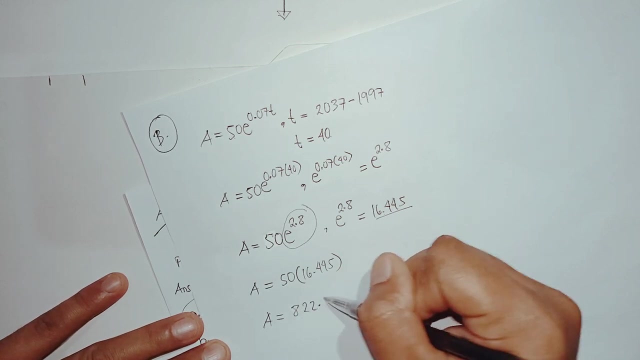 so it is 16.445. now let's plug in this here to continue. we have a- is equal to 50 times the value of this one, which is this: okay, 16.445 now. 16.445 times 50 is equal to 822.25. okay, so let's go back.